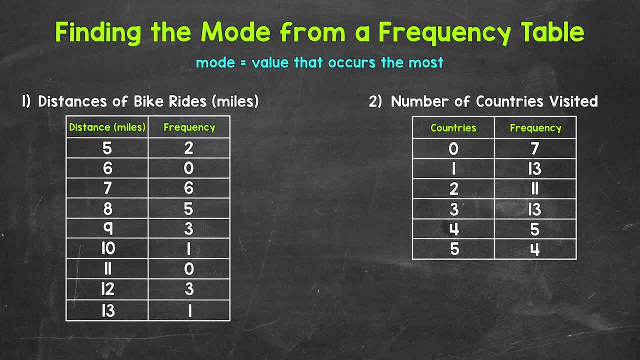 occurred the most. Well, if we look at our frequency table, five miles occurred twice. six miles occurred zero times. seven miles occurred six times. eight miles occurred five times. nine miles occurred three times. ten miles occurred once. eleven miles occurred zero times. twelve miles occurred three times. 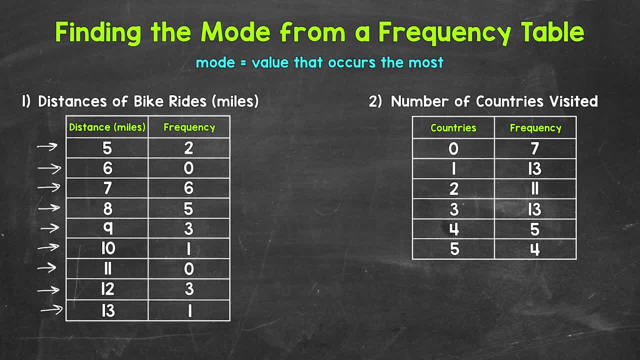 and thirteen miles occurred once. That means that seven miles occurred, the most 6 times. So our mode is seven And we can label this miles. So the most frequent distance, the distance that occurred the most, was seven miles. So that's our mode. Let's move on to number two, where we have 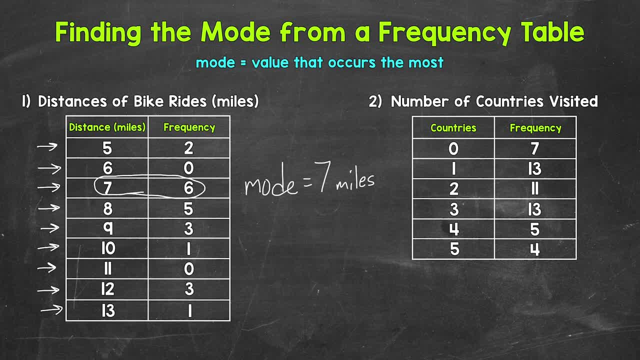 a frequency table displaying the number of countries visited, and these are the countries outside of the country you were born in. So let's say that a group of people were asked the number of countries they have visited outside of the country they were born in. These are the results. 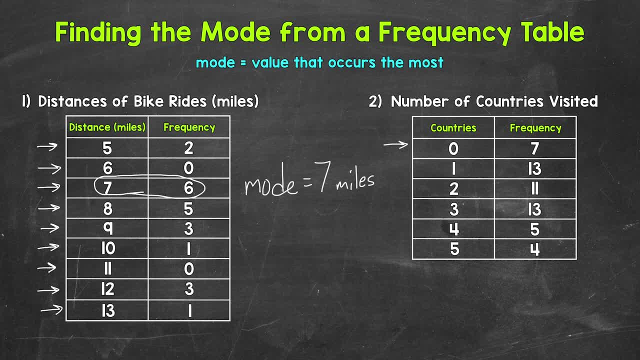 So zero countries seven people, One country 13 people, Two countries 11 people, Three countries 13 people, Four countries five people And then five countries four people. So it looks like one country occurred 13 times and three countries occurred 13 times. So those two values. 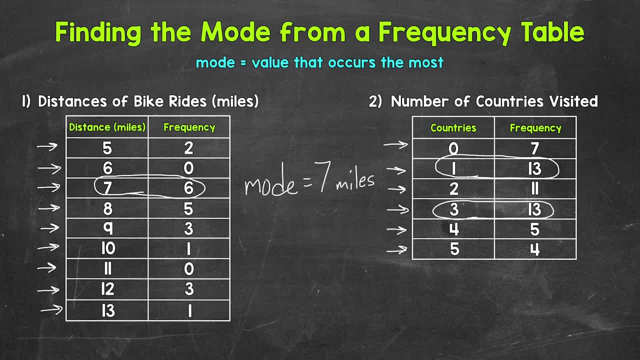 are the number of countries that were visited outside of the country they were born in occurred the most. So we have two modes here. Our modes are one and three countries. So one and three countries visited occurred the most. So if the data set works out to where there, 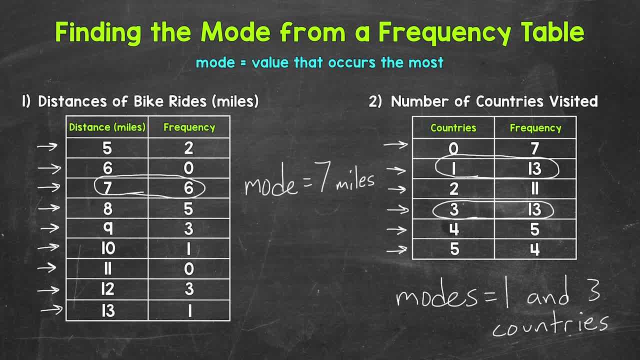 is more than one mode, that's perfectly okay. So there you have it. There's how to find the mode from a frequency table. I hope that helped. Thanks so much for watching. Until next time, peace.